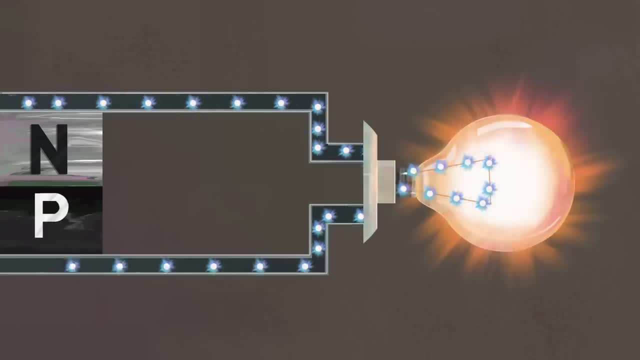 directed by thin metal fingers at the top of the cell. From there they flow through an external circuit, doing electrical work like powering a light bulb, before returning through the conductive aluminum sheet on the back. Each silicon cell only puts out half a volt. 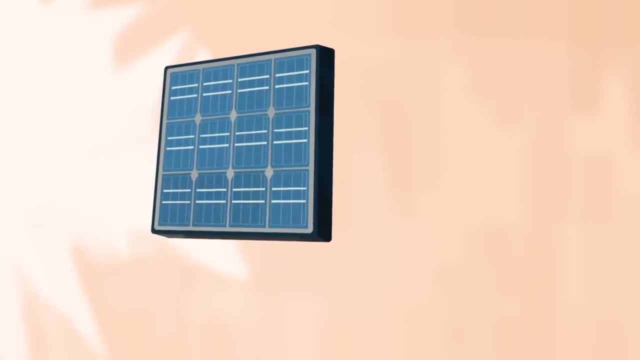 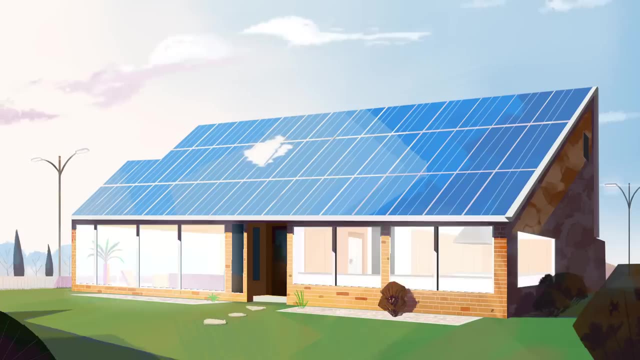 but you can string them together in modules to get more power. Twelve photovoltaic cells are enough to charge a cell phone, while it takes many modules to power an entire house. Electrons are the only moving parts in a solar cell, and they all go back where they came from. 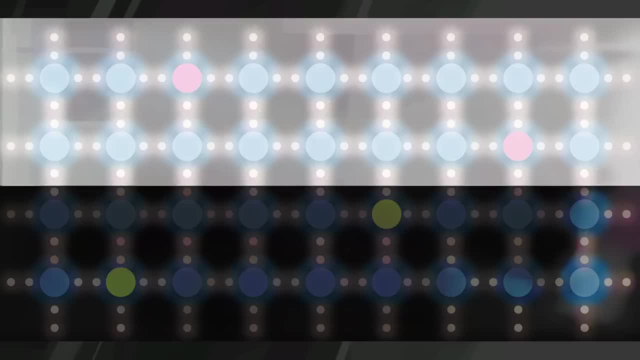 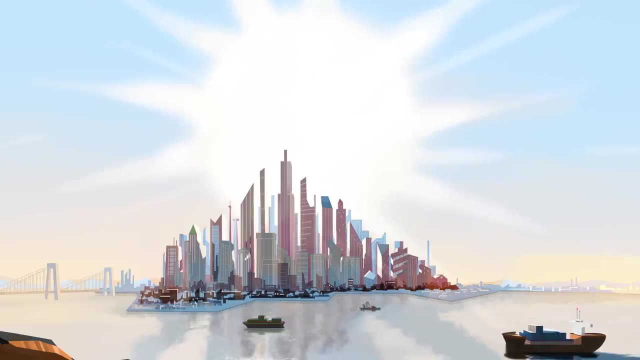 There's nothing to get worn out or used up, so solar cells can last for decades. So what's stopping us from being completely reliant on solar power? There are political factors at play, not to mention businesses that lobby to maintain the status quo. 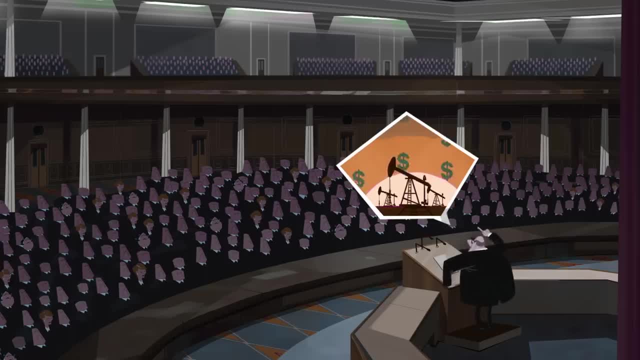 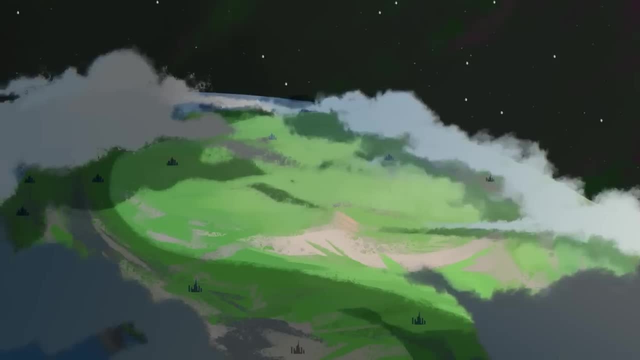 But for now, let's focus on the physical and logistical challenges, And the most obvious of those is that solar energy is unevenly distributed across the planet. Some areas are sunnier than others. It's also inconsistent. Less solar energy is available on cloudy days or at night. So a total reliance would require efficient ways to get electricity from sunny spots to cloudy ones, and effective storage of energy. The efficiency of the cell itself is a challenge too, If sunlight is reflected instead of absorbed, or if dislodged electrons fall back into a hole. 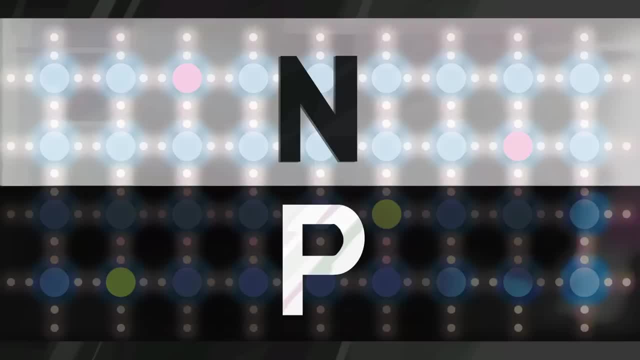 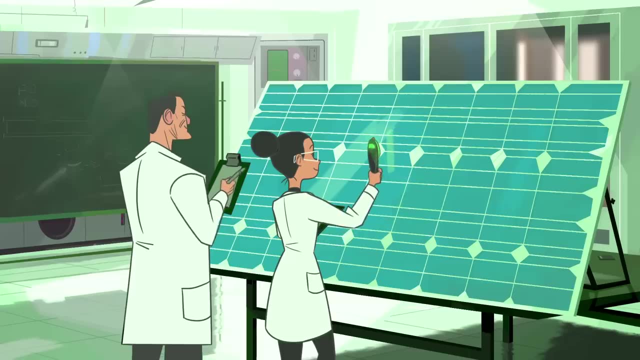 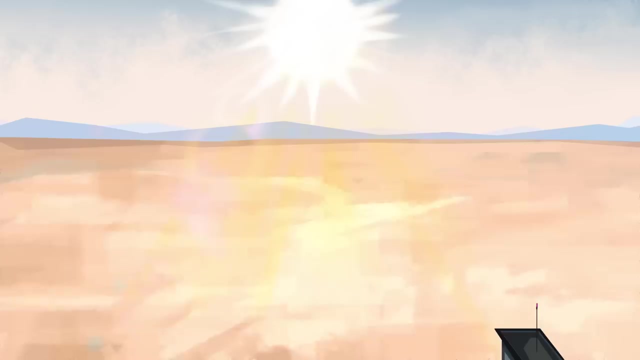 before going through the cell, that photon's energy is lost. The most efficient solar cell yet still only converts 46% of the available sunlight to electricity, And most commercial systems are currently 15 to 20% efficient In spite of these limitations. it actually would be possible to power the entire world with today's solar technology. We'd need the funding to build the infrastructure and a good deal of space. Estimates range from tens to hundreds of thousands of square miles, Which seems like a lot. 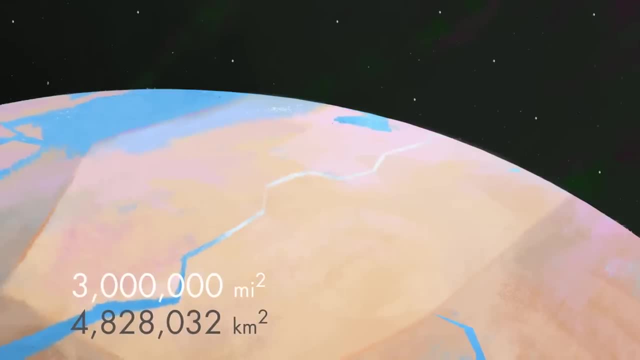 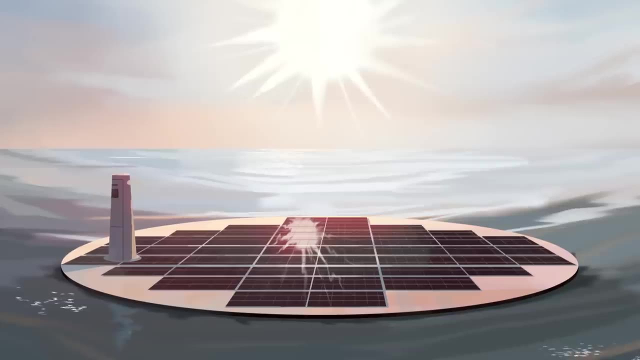 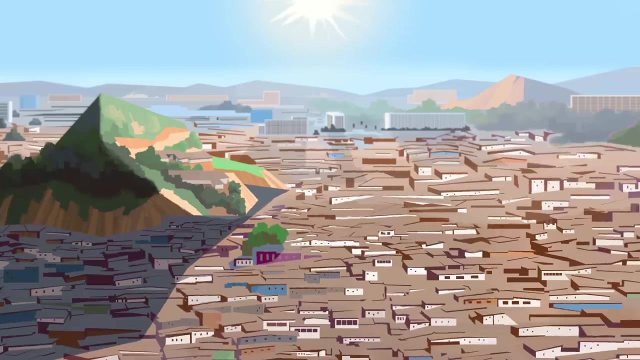 but the Sahara Desert alone is over 3 million square miles in area. Meanwhile, solar cells are getting better, cheaper and are competing with electricity from the grid, And innovations like floating solar farms may change the landscape entirely. Thought experiments aside, there's the fact that over a billion people don't have access to a reliable electric grid, especially in developing countries, Many of which are sunny. So in places like that, solar energy is already much cheaper and safer than available alternatives like kerosene For, say, Finland or Seattle, though. 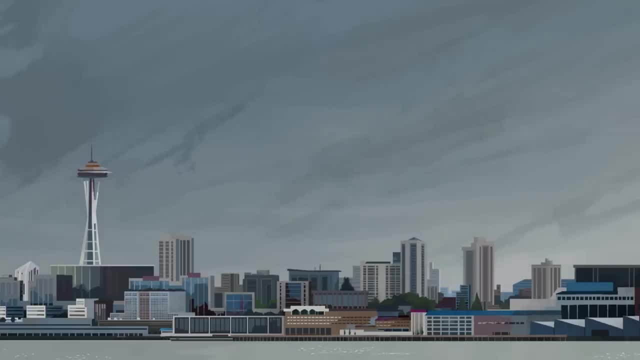 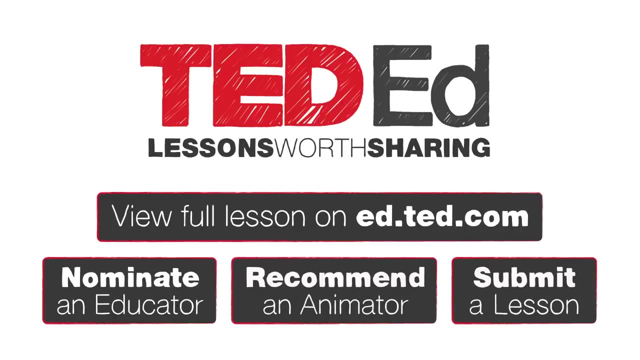 effective solar energy may still be a little way off. For more UN videos, visit wwwunorg.